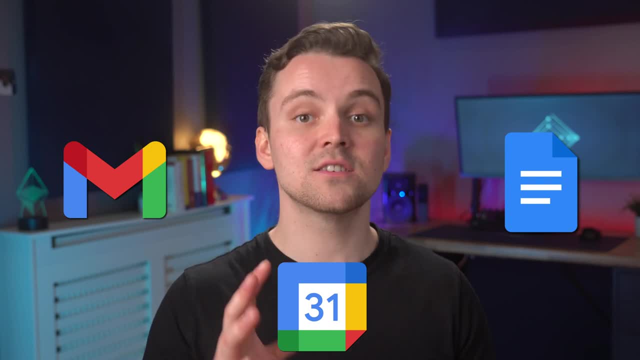 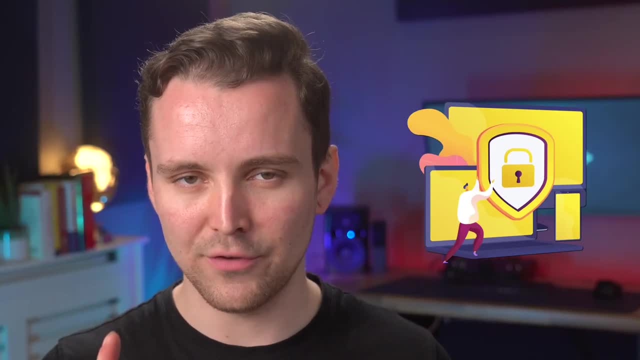 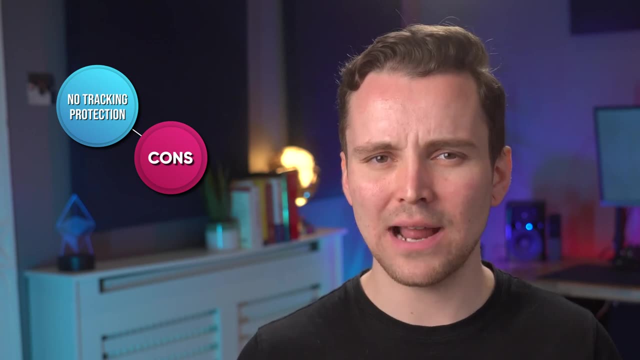 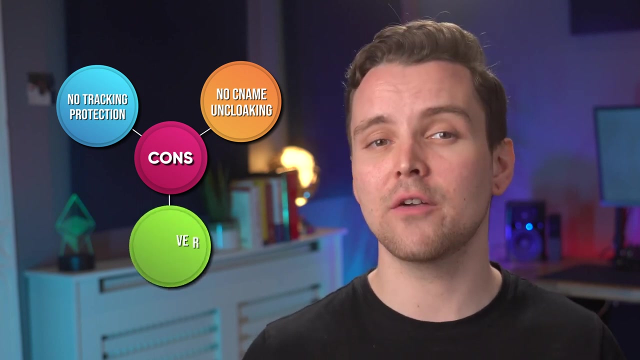 easier with its concise bookmarks bar. When it comes to your privacy, however, Chrome has a few shortcomings. It has no tracking protection or ad blocking for any compatible platforms unless you download a third-party extension. No C-name uncloaking to block first-party ads and offers you very little control over. 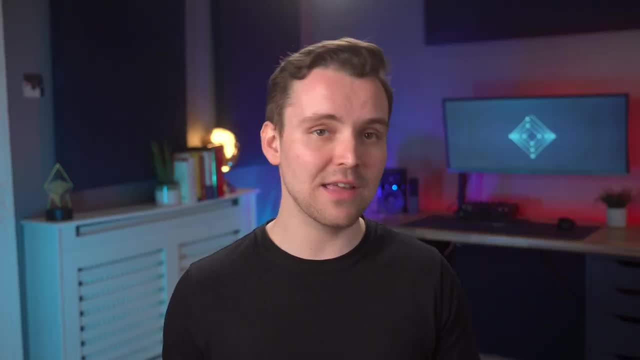 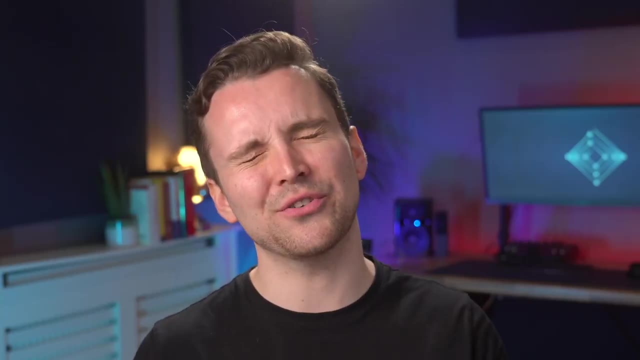 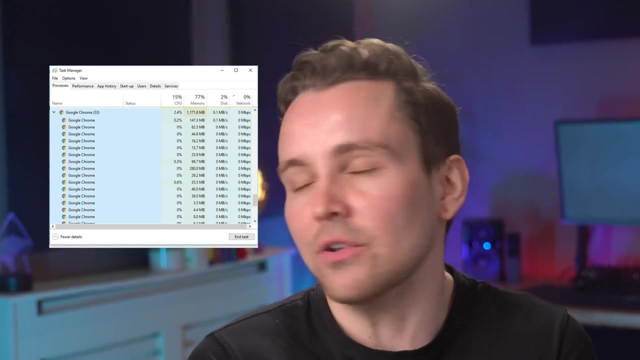 website permissions. Basically, Google is going to do whatever they want with your private information, and there's nothing you can do about it. If you're running Chrome on a low-end device, brace yourself for spontaneous combustion. This browser is an absolute nightmare when it comes to system impact, but you probably already know that. 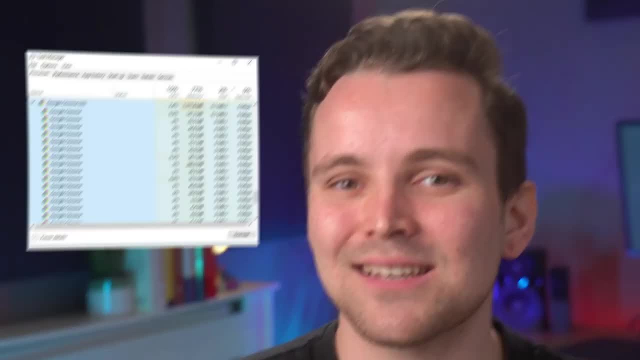 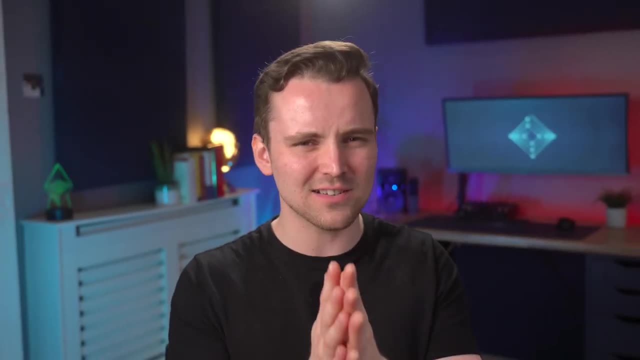 Sorry, that was probably your RAM, but you probably already know that, Overall, Chrome is great for the working man, thanks to its full suite of apps and excellent synchronization, but we can't just overlook the glaring privacy issues. For this reason, we're putting it in the decent tier. 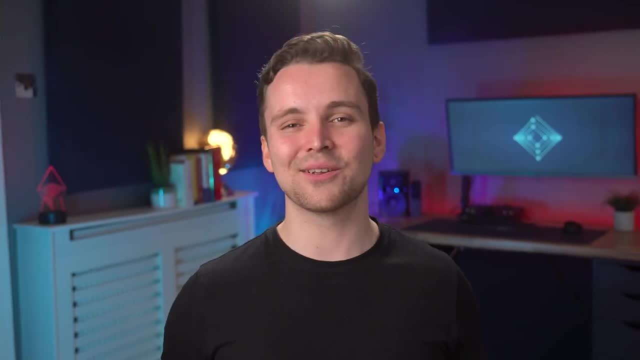 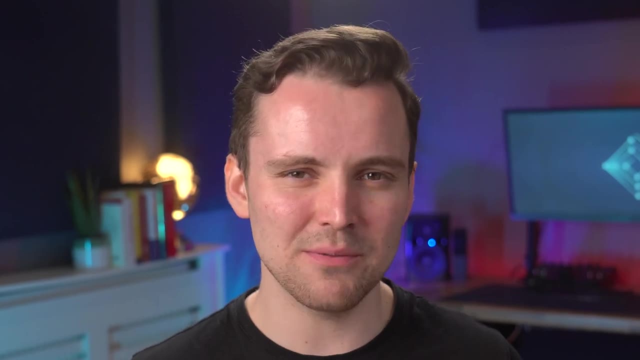 Next up, Microsoft Edge, What we oldies like to call Internet Explorer. Microsoft Edge has evolved into one of the best web browsers in the world, And it's honestly such a shame that most people don't use it. Look how far you've come. You've made me so proud. 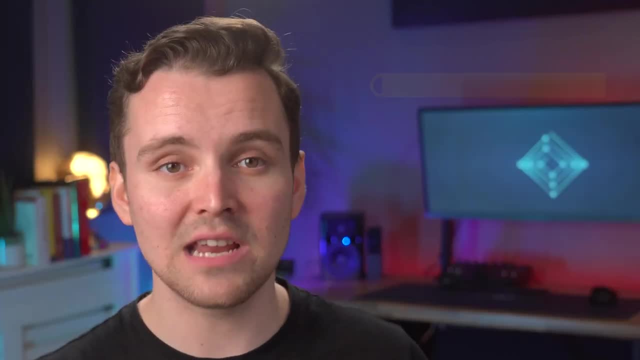 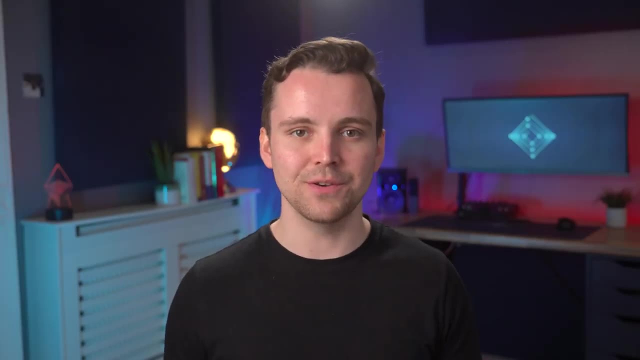 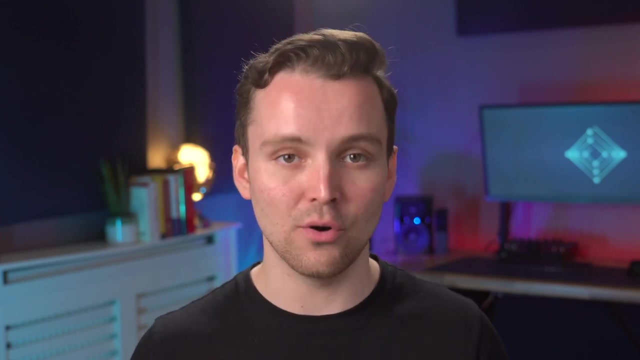 The browser has become a titan of privacy, with tracking protection across all platforms, robust ad blocking and allowing you to clear cookies on exit. As for synchronization, Edge rivals Chrome with its password and bookmark syncing, history and open tab syncing, and end-to-end encryption of your synchronized data. 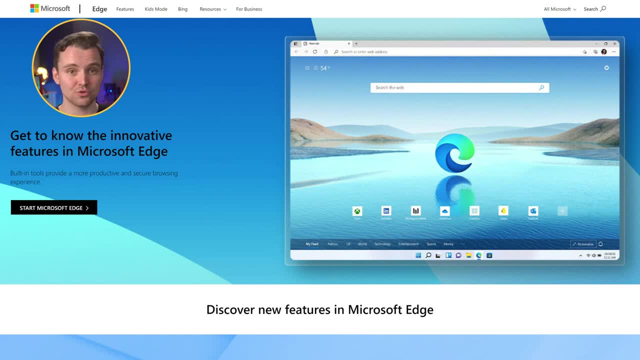 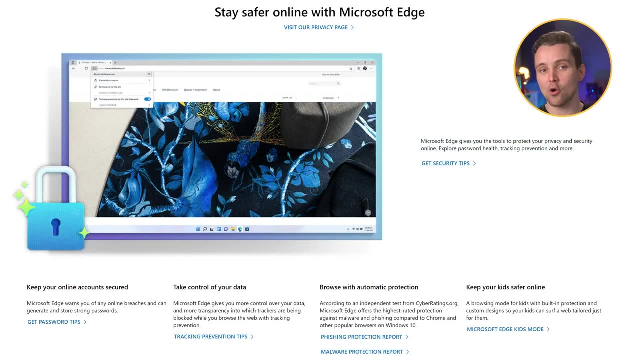 Edge ups its game further with its significantly lower resource drain, which means that your computer isn't going to combust if you open too many tabs. The browser features a wide range of robust privacy features that help keep those nosy websites at bay, and Microsoft made sure to stay well away from flops. 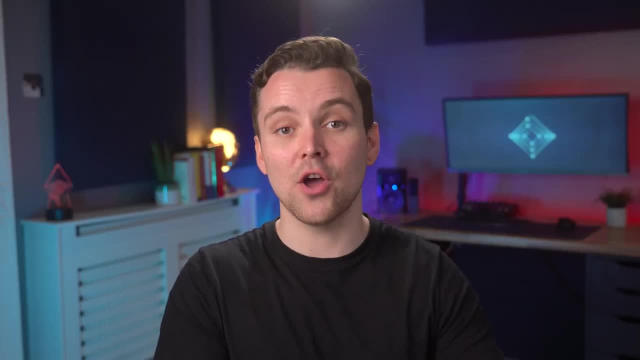 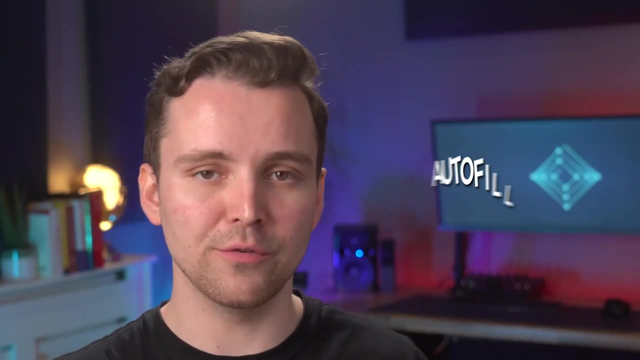 Google's current solution for ad targeting in the absence of third-party cookies. unlike Chrome, It's got a full range of convenience features like autofill, website translation, dynamic text reflow and more, If you're sick of Chrome compromising your privacy. 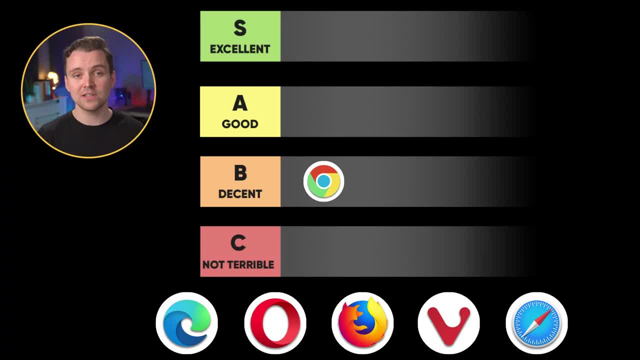 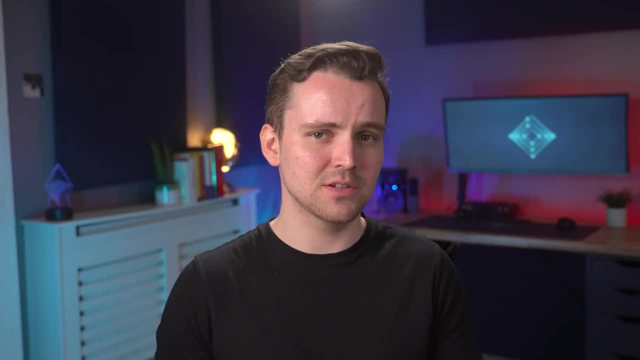 Microsoft Edge is a fantastic alternative and for this reason, we're placing it in the good tier. Next, let's take a look at Opera. Opera is not a very well-known browser, despite being one of the top five browsers used around the world, But if you're a gamer, then you should definitely consider switching. 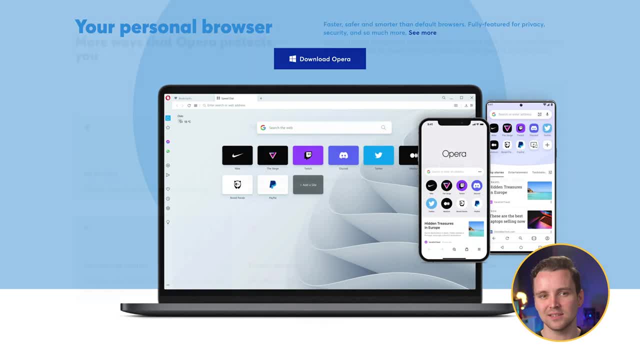 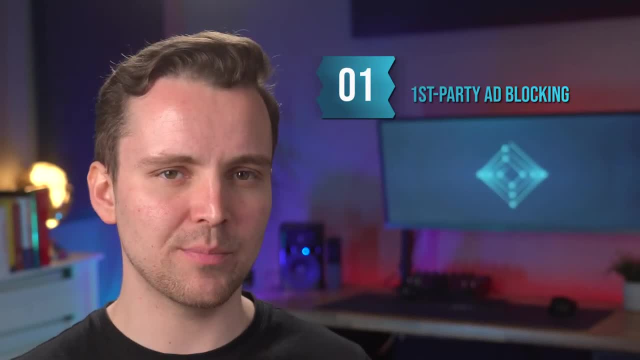 to Opera thanks to its light performance impact on all devices. In the privacy department, Opera provides tracking protection and integrated ad blocking, but that's about it. Don't expect any first-party ad blocking, cookie clearing on exit or JavaScript and hyperlink auditing or ping disabling. 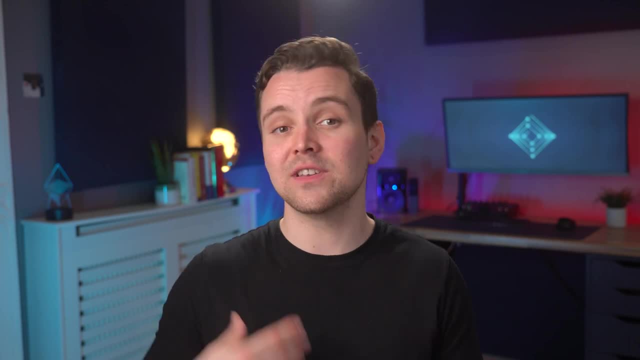 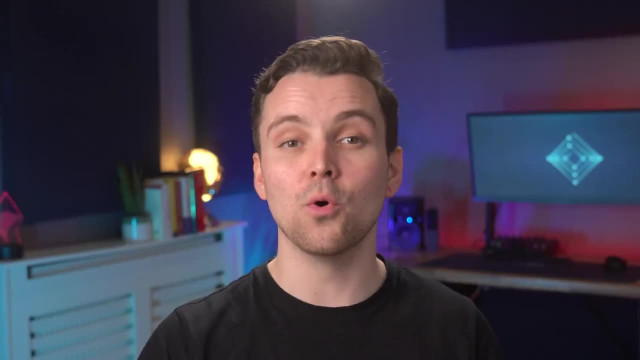 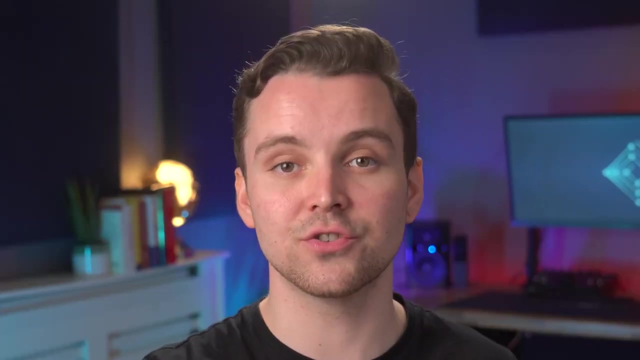 even with extensions, However, the browser redeems itself with its synchronization, and you'll be able to sync all of the important stuff across your devices, like your passwords and bookmarks. What's more, Opera offers full extension support, with support for uBlock, Origin extension, sideloading and its own extension store for you to browse when you're. 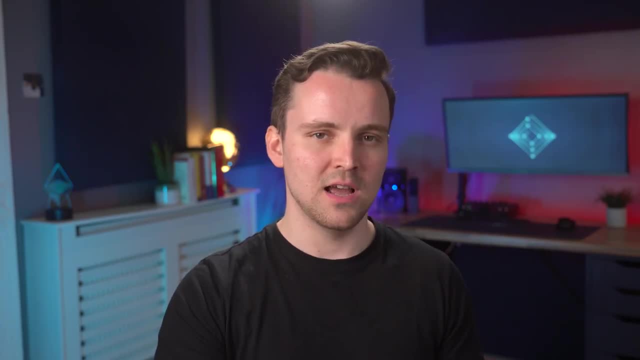 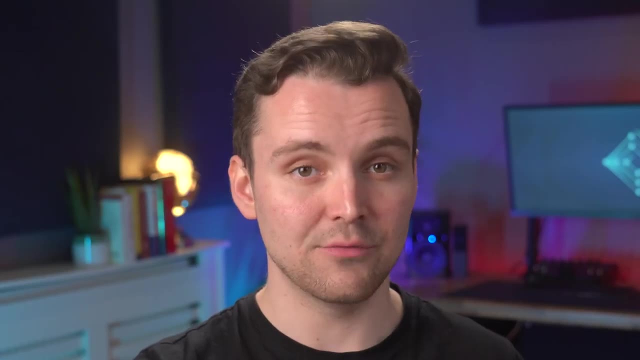 bored of regular shopping. Simplicity is where Opera shines, and while it doesn't offer a lot of privacy options, it's not going to siphon your personal data and set it off to the highest bidder. For that reason, and the fact that its light memory load makes it great for gamers, 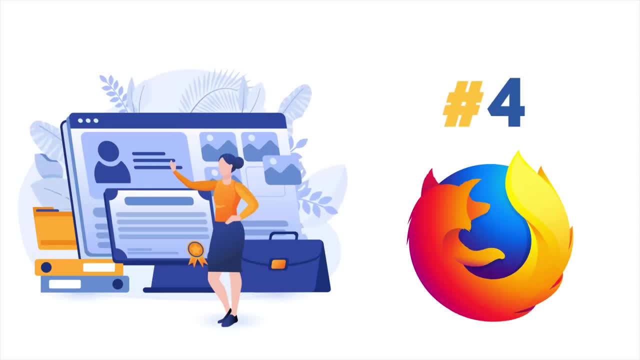 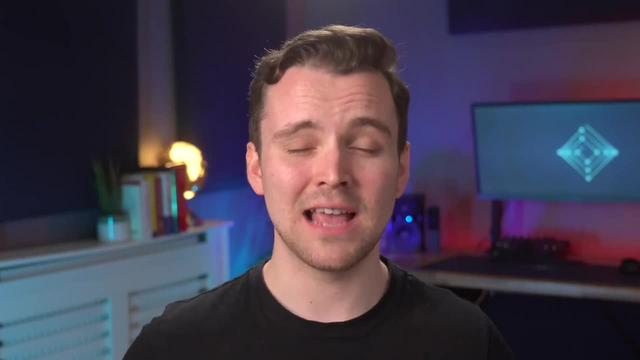 we're putting Opera in the good tier. Up next is Mozilla Firefox. I believe you've already been introduced. There we go. Mozilla Firefox has become a browser to be reckoned with, and while I'm not particularly fond of the simplification of the icon, 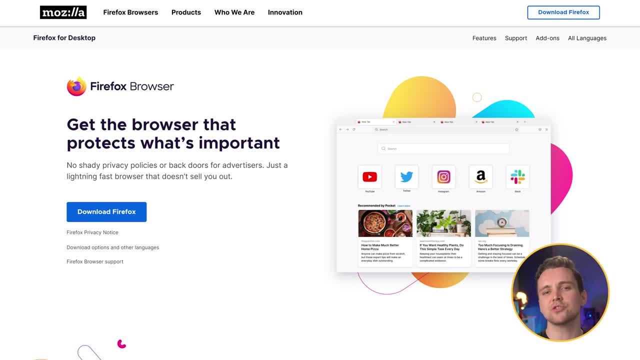 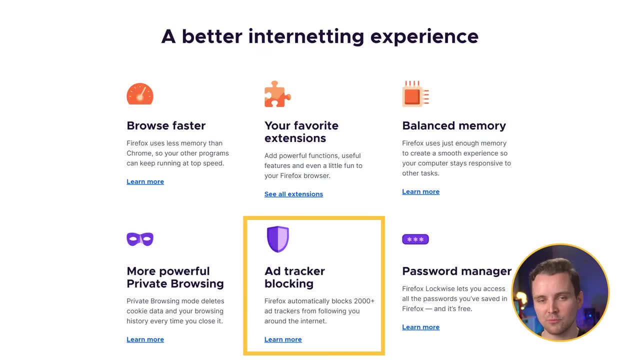 everything else about this browser is excellent. The revitalized version of Firefox now has a much lighter impact on your computer, using far less RAM than before. It offers total tracking protection across all platforms, as well as the ability to clear cookies on exit and. 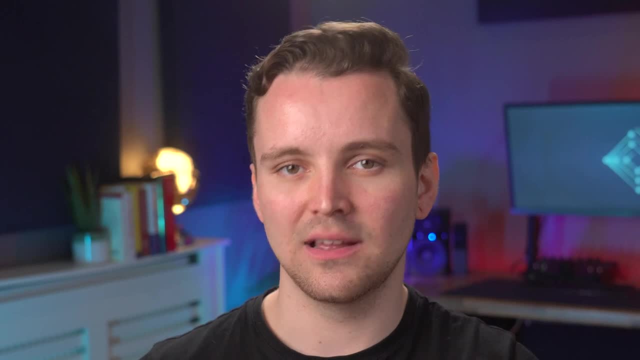 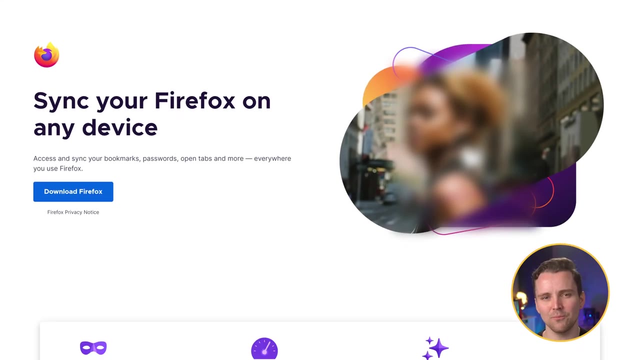 third-party storage, While it doesn't offer its own ad blocking. downloading a simple extension is a piece of cake and it should feel familiar if you're transitioning from Chrome. It's got brilliant synchronization as well, with full bookmark, password history and setting. 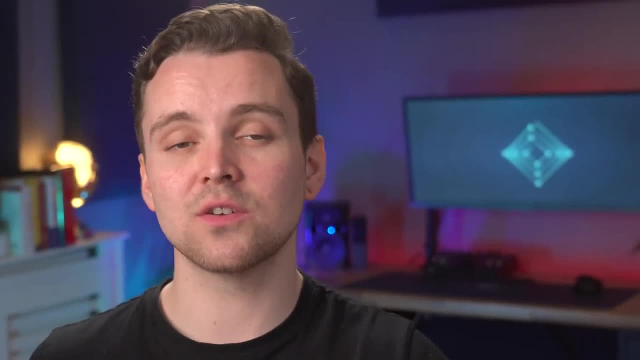 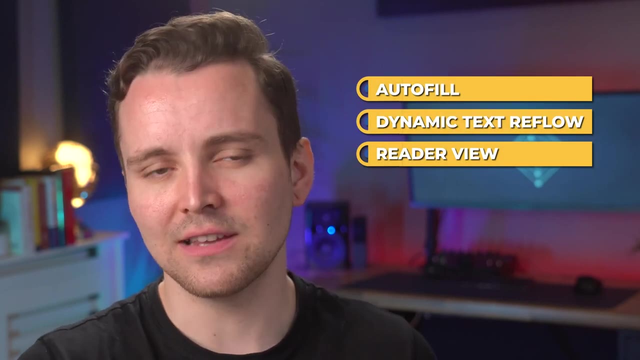 synchronization across all platforms. As for convenience, when you're on desktop you'll have access to autofill, dynamic text reflow and reader view, though Mozilla is also in the experimental stage with website translation and dark mode. Mozilla Firefox is the king of. 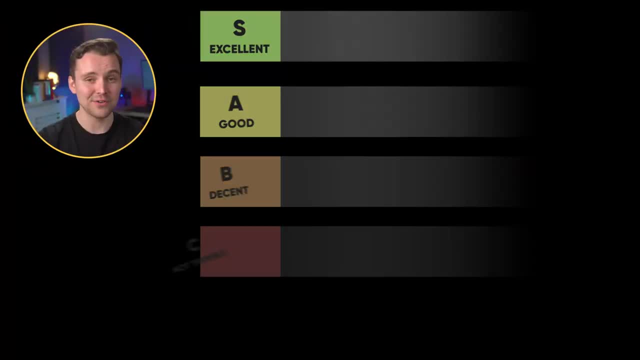 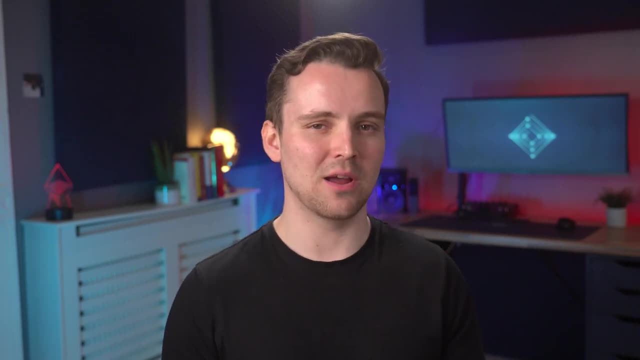 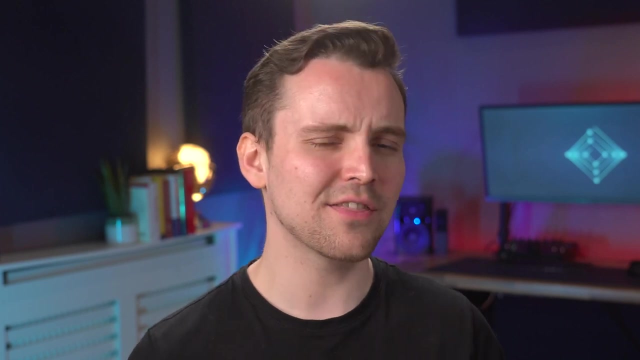 privacy, synchronization and convenience, and for that reason we're placing it in the excellent tier. Take that Chrome. We've got another obscure browser coming in people. Vivaldi is here. I hate to disappoint all of the classical musicians, but the Vivaldi browser has nothing. 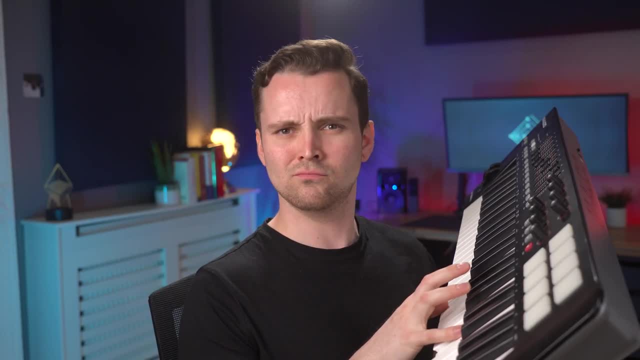 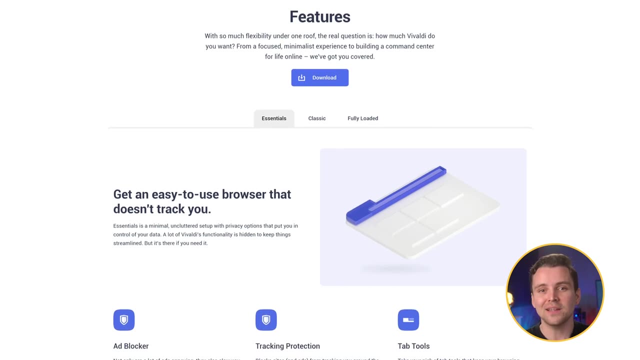 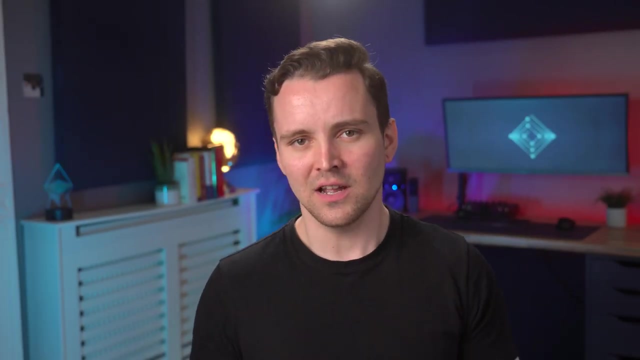 to do with the baroque composer? Aww, really. What it does have, however, is a few great features. It's a spin-off of Opera taking the best of its parent browser and pushing the limits of customization. This is a browser that is loaded with features. 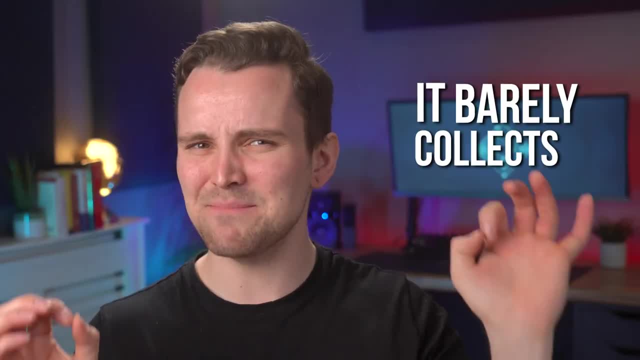 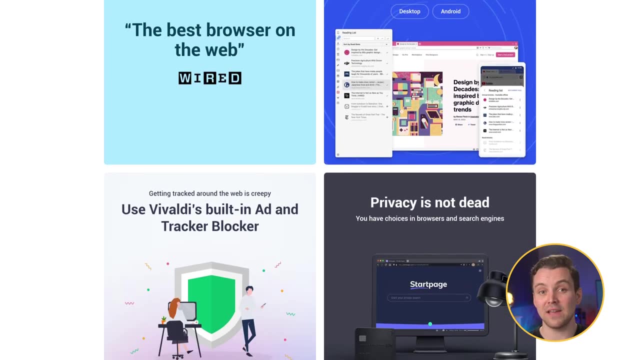 that you would normally have to download in an extension and, the best part, It barely collects any data. The Vivaldi browser is intended to be a fully-featured customizable browser without the need for any extensions, though if you did want to download some extensions, you'd be able. 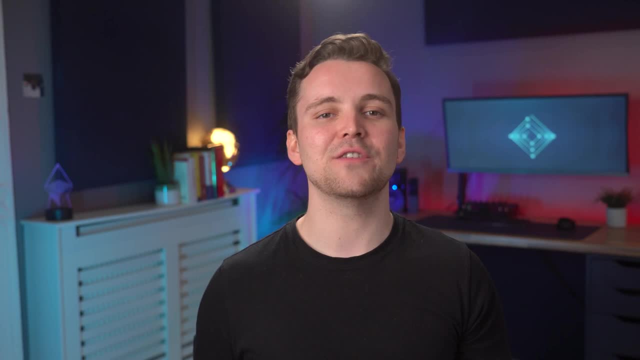 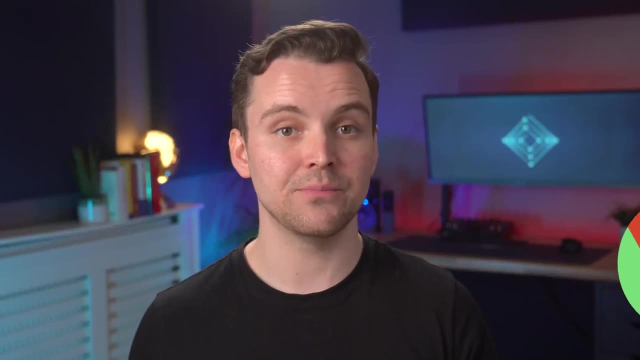 thanks to its Chromium foundations. Not only does Vivaldi feature an abundance of features right out of the box, but it also has a low RAM consumption, so it's not going to slow down your machine if you have more than three tabs open. Yep, Yep, I'm talking about you. 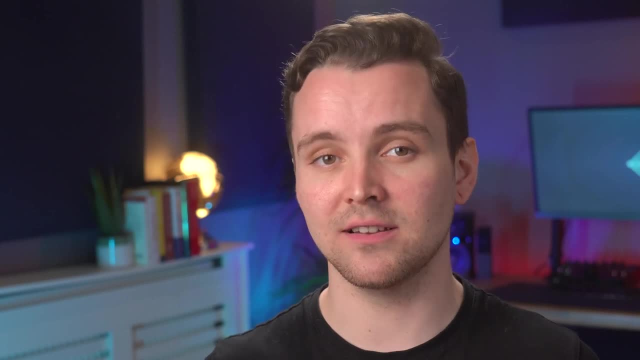 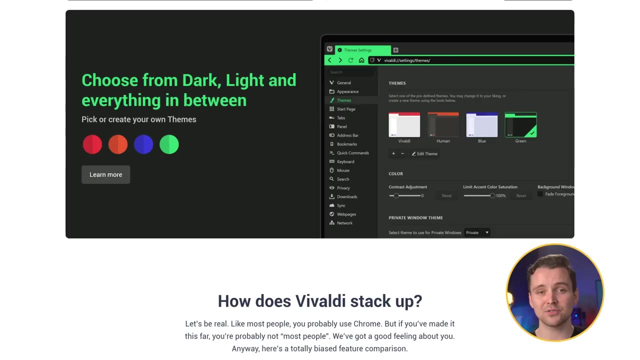 By creating a Vivaldi account, you'll be able to synchronize your settings and browser data across your other devices, offering a seamless experience. Another cool feature from Vivaldi is that the browser offers themes which you can change at your leisure and even set to switch at certain times. 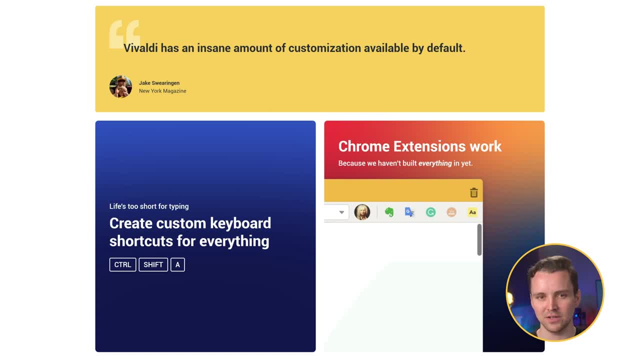 If you're a power user who wants a lot of customization in their browser and doesn't mind a little bit of ethical data collection, then Vivaldi is the place for you. If you're a power user who wants a lot of customization in their browser and doesn't mind a little bit of ethical data collection, then Vivaldi is the place for you. 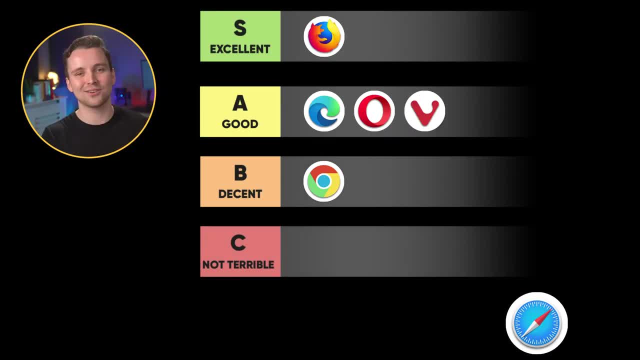 If you're a power user who wants a lot of customization in their browser and doesn't mind a little bit of ethical data collection, then Vivaldi is the place for you. We're placing it in the good category for this one And for all you die-hard capitalists- I mean Apple lovers. 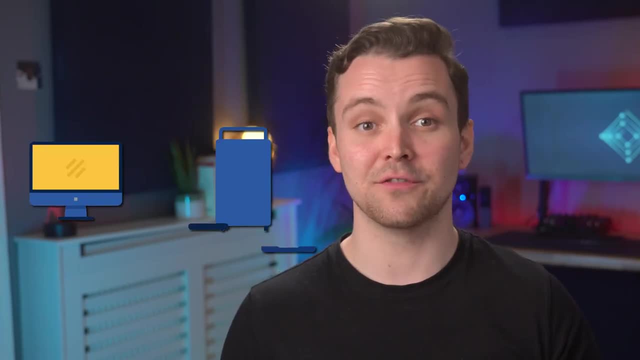 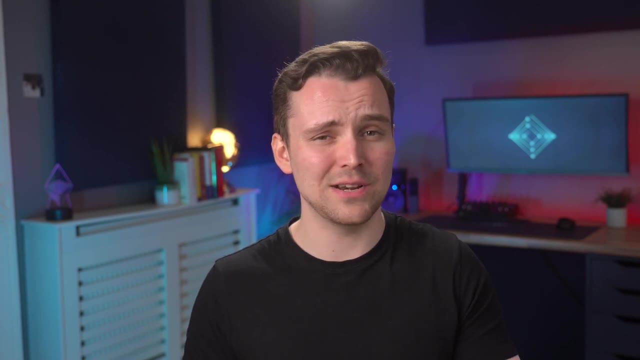 Safari is up next. Safari is the native browser for all Apple's devices. If you've got an iPhone, you've probably used it at least once. It's not exactly the best browser in the world for a lot of reasons. For one, it literally is only usable on iOS devices. 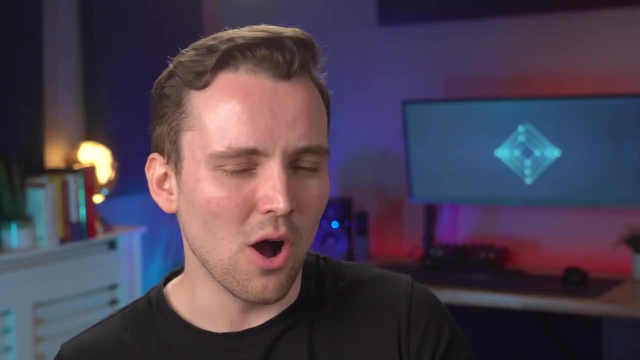 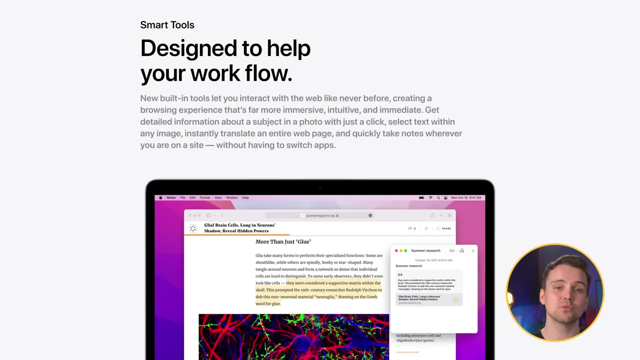 So even if you really like Safari- which you might not after watching this video- you wouldn't be able to use it without an Apple device. Safari isn't all bad, though. Apple is also on top of their synchronization game with the ability to sync bookmarks.